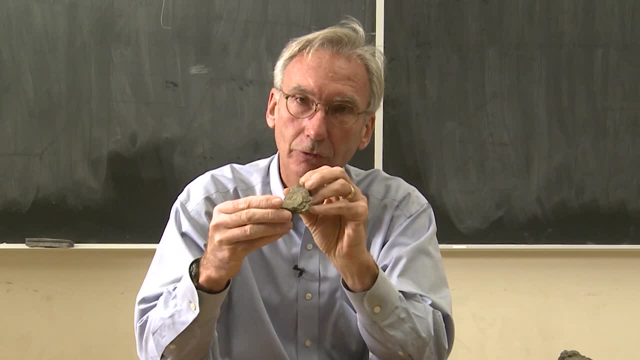 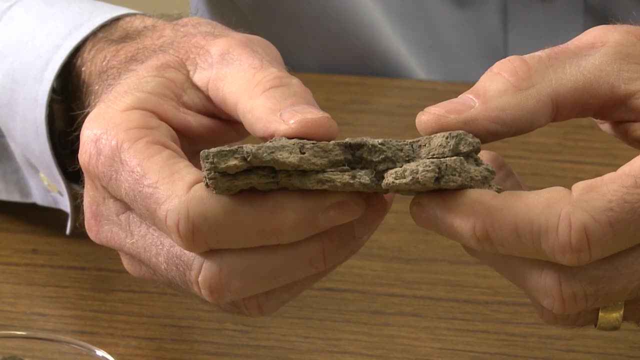 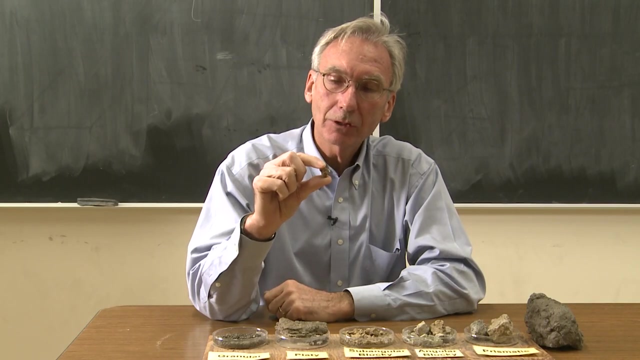 And actually you can get platy structure to form in your soil by the type of tillage practice that you do. You do a lot of moldboard pawing or conventional tillage. you're going to get the formation of platy structure. So in the B horizon we actually have two types of 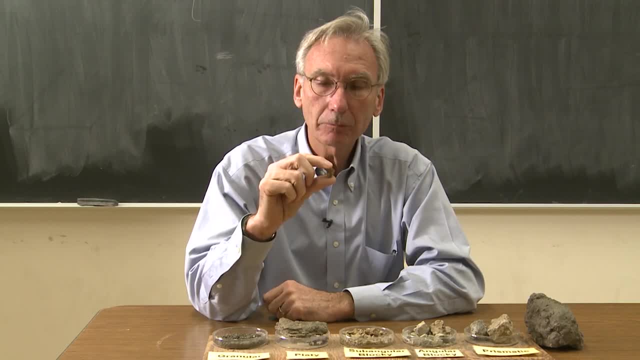 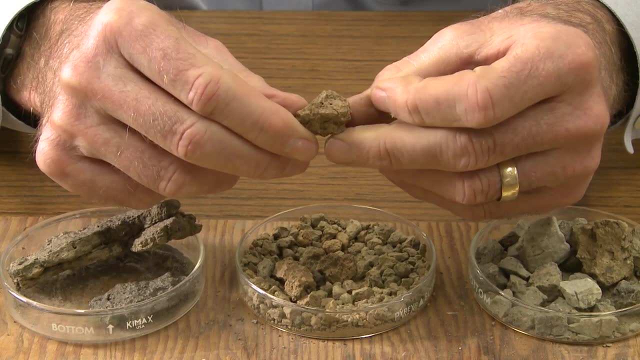 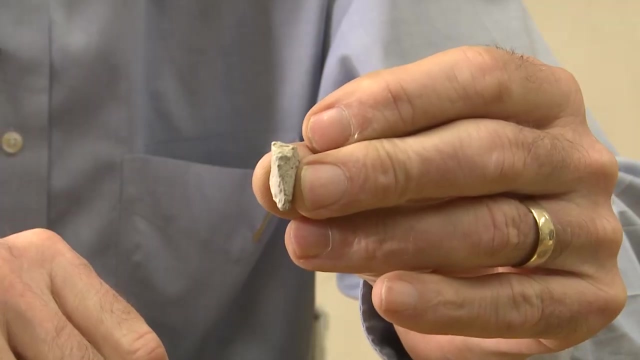 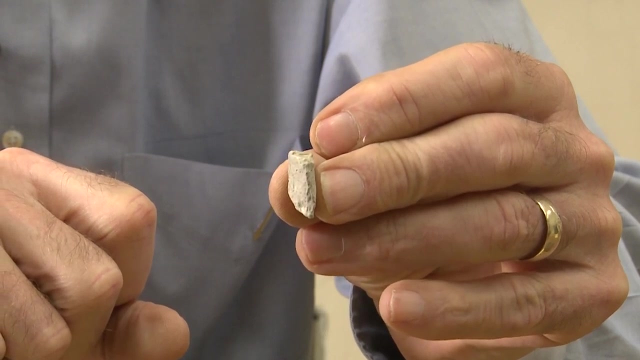 structure. We have what is called subangular blocky structure and angular blocky structure, And with subangular blocky structure the edges of the blocks are actually rounded off, versus angular blocky structure, where you have these sharp angles which occur in the blocky structures. 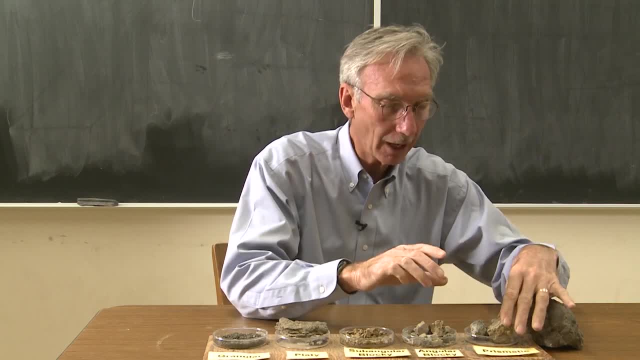 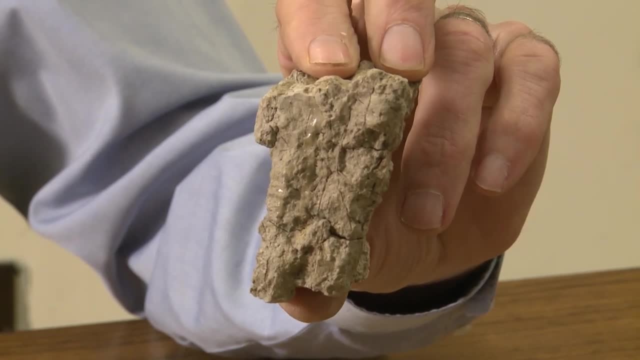 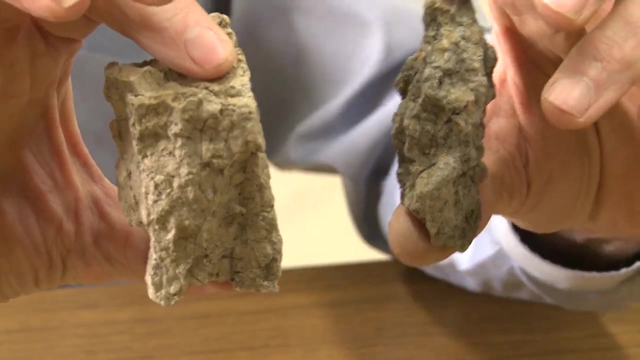 Also in the B horizon you could have what is called prismatic structure, And prismatic structure is long in the vertical direction, sort of short in the horizontal. it's got sharp edges. You can also have prisms that are smaller. You can have small. 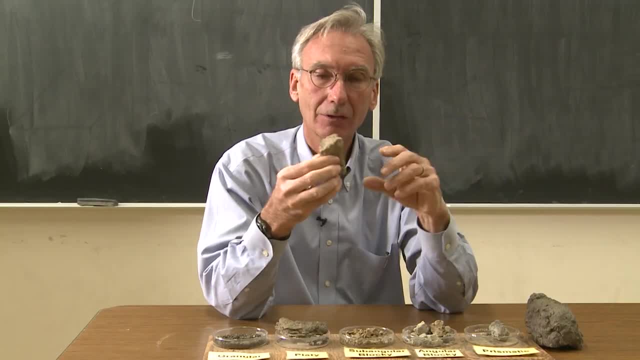 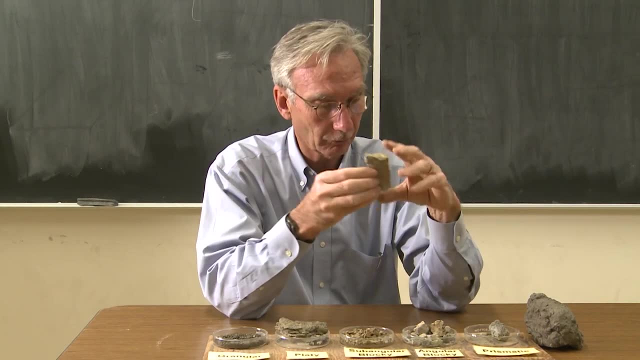 prisms. you can have large prisms. The size of the structural unit is pretty irrelevant, because you can have all sorts of different sizes for these different types of structures. The other type of structure that we have in the B horizon is something called cladding. Cladding is a type. 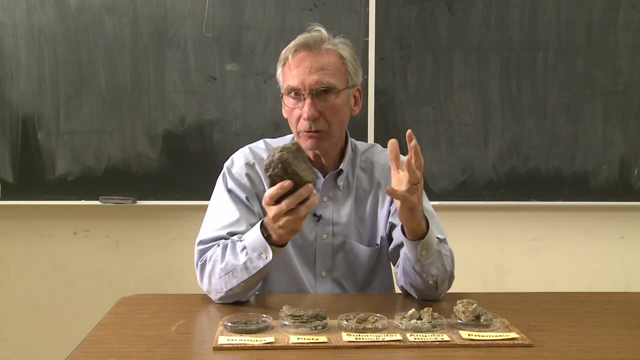 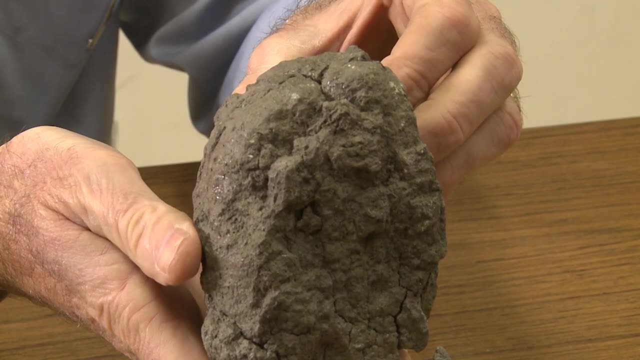 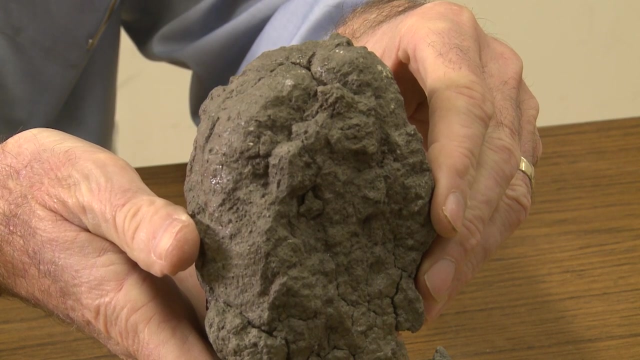 of structure called columnar structure, And columnar structure is not so common here in Indiana, but we do see it. It's where you have a lot of salt in your soil and what happens is that the salt causes the tops of the prisms to disperse and so to round off and you end up. 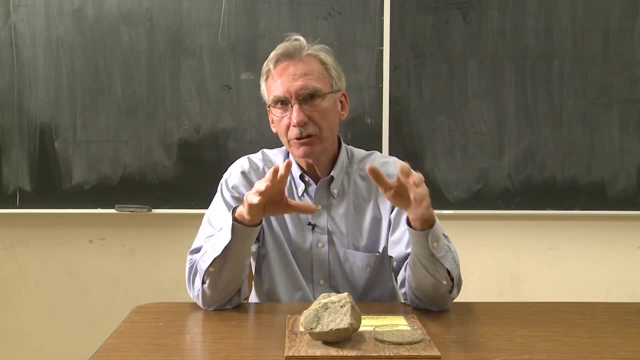 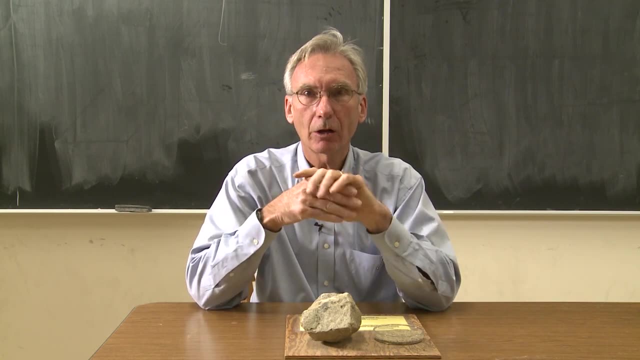 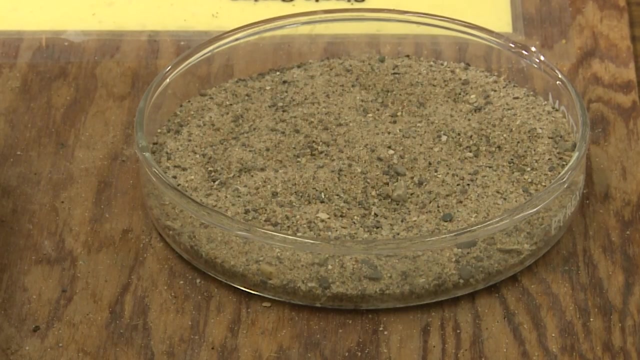 with what's called columnar structure. What's the situation down in the C horizon, where the parent material is? Actually, we do have what is called units in the C horizon, And usually that consists of sand. sand or it consists of a massive 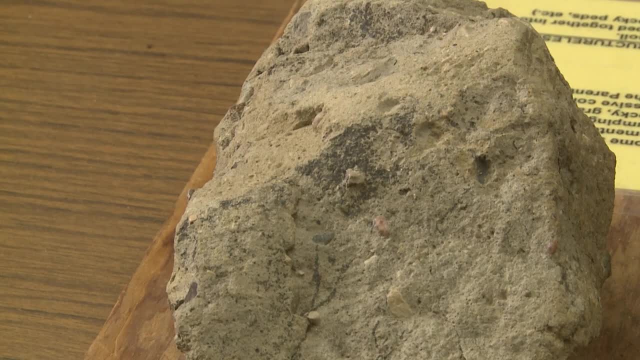 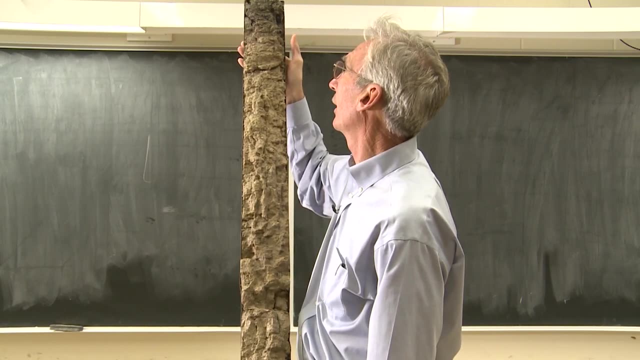 type of structure, Everything just kind of glued together. So let's conclude by looking at the soil structures in a soil monolith or a soil profile. Top of the soil profile, the A horizon, that's where you find granular structure. In the